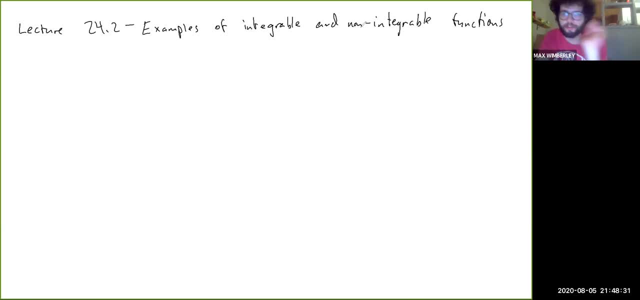 Okay, so in this video we're gonna look at some examples of using this definition we just made of the integral, the d'Arbu integral. So for the first one. so let's see, say f of x is x squared and we're integrating it on the interval zero b. 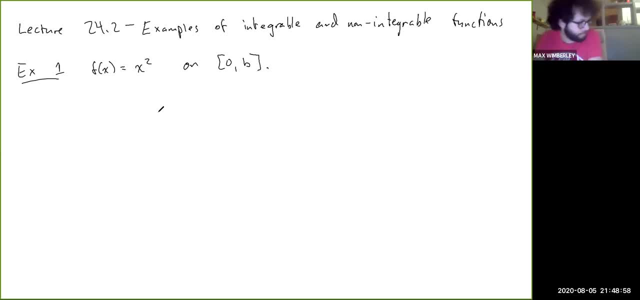 Okay. so of course we know what we expect the answer to be, but we're trying to see how we can get there using the definition we just made right. So consider p partition to be right. well, okay, So first. okay, let's give the formula here. So for a partition. sorry, 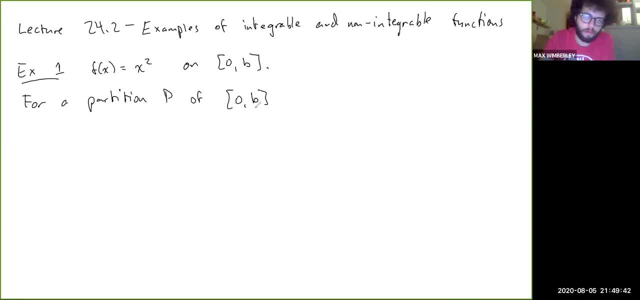 p of zero b. we have that. the upper sum of f on p is the sum from here between y and z square root 2 times minus The very opposite. It's a slight deviation, Okay. so theorie of an inflection can be as follows: So ducking is f x square root 2 times 1, right f means 1, because n equals 1 to n of m f, tk minus tkring 1, or because y equals 1, 2n of m F, tk for tk or tk minus 1, tk times tk minus 1, orth vontade escape cheers. 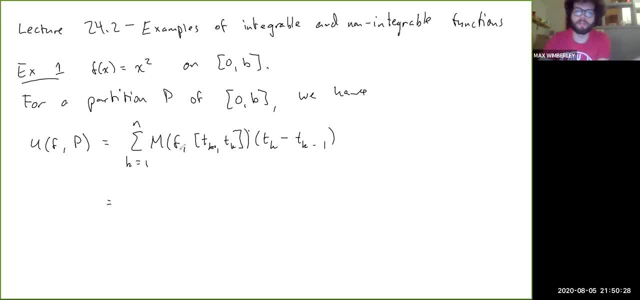 non-negative and x squared is increasing, so it actually achieves its maximum value on this interval. the maximum value is just TK squared, right? so it achieves that when X equals TK. so this is: the sum from K equals 1 to n of TK squared, TK minus TK minus 1. okay, so right suppose for some n we choose P by setting TK. 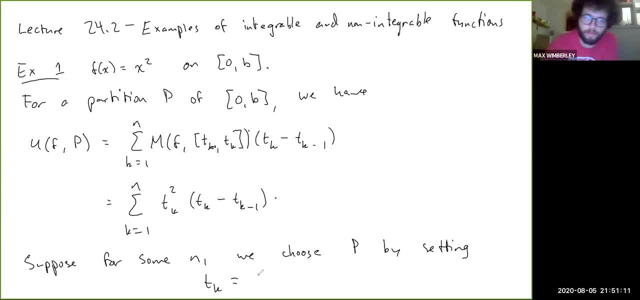 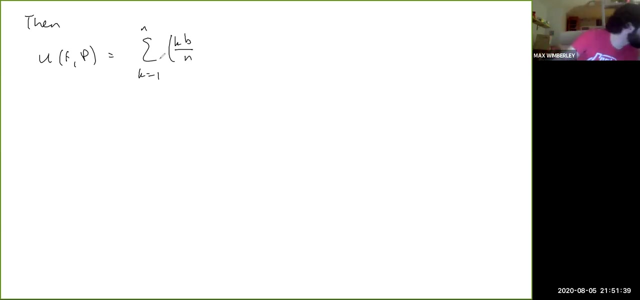 equals KB over n right. so this is like the equally spaced partition, equally spaced partition right. then UFP, using our formula, is: the sum from K equals 1 to n of KB over n right. squared times KB over n minus K minus 1, b over n, which is the sum from K equals 1. 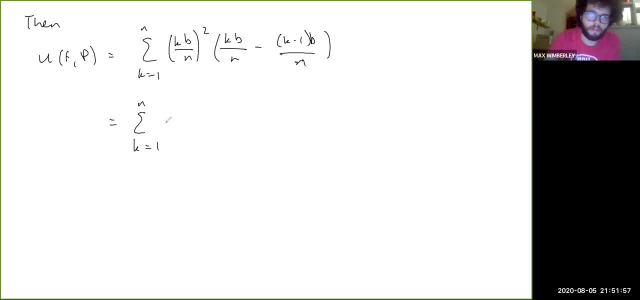 to n. okay, let's say, yeah, K squared, b squared over n squared times, and then we have 1 over n here, or b over n, sorry. and so if we just factor out about b over b, cubed over n cubed, we get b cubed over n cubed. sum from k equals one to n of k. 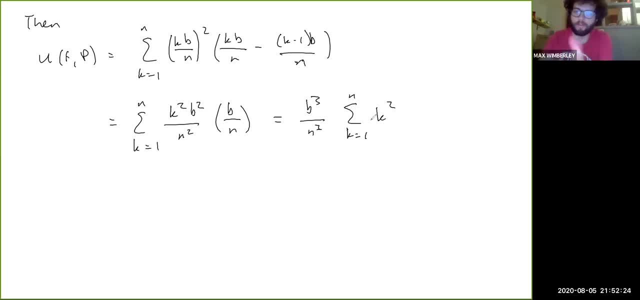 squared, and there's just a formula. there's just a formula for the sum of of squares from one to n. so we get b cubed over n cubed times n times n plus one times two, n plus one over six, right, so um, so u of f is less than or equal to: 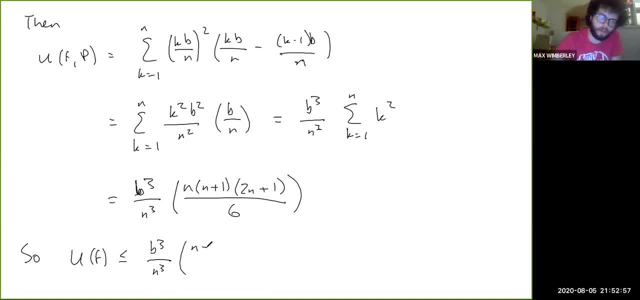 b. cubed over n. cubed times: n oops. n. n plus one, two n plus one over six, which tends to, as n approaches, infinity. this tends to be cubed over three. right, because on top here we have a cubic polynomial in n whose highest degree term is two. n cubed right. 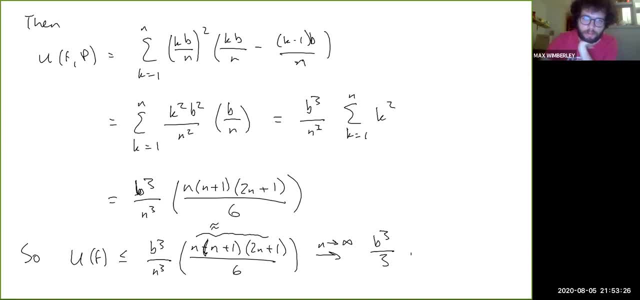 so. so this is, like you know, asymptotically governed by two n cubed on top right, and then we have n cubed on the in the denominator six, n cubed in the denominator right. so this is a pretty simple limit to evaluate. so, as n approaches infinity, this is b cubed over three. 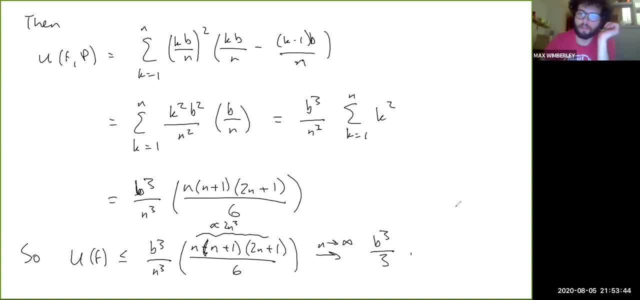 so u of f should be less than or equal to b cubed over three. so u of f is less than or equal to b cubed over three. right, because u of f is the infimum of all of the um, u of fp, right. so it's like, well, all we're doing is, it's just, we know. 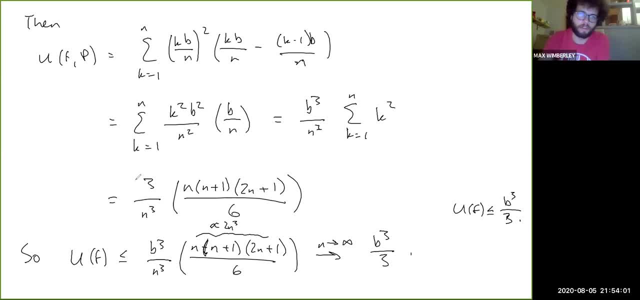 a very we know like a special sequence of partitions that we're sure is gonna make u of fp approach the correct value. so by using that special sequence of partitions we can like sort of find the correct value and show that, like u of f is less than or equal to that value. 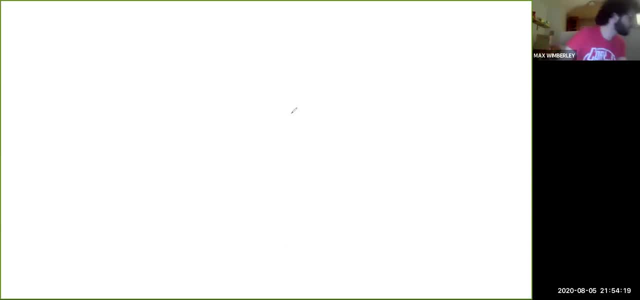 and then similarly right. so, so, similarly, um, l of fp equals, like the sum for l of fp, you end up using the left endpoint because that's the smallest value on the integral, on the interval, sorry, the subintervals. so we have the sum from k equals n or k equals one to n of. so the left endpoint is k minus one squared, b squared, sorry. 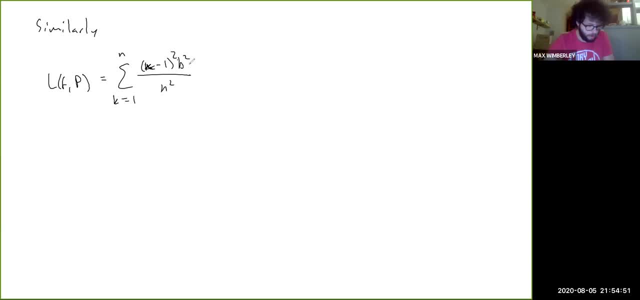 k minus one squared b squared over n squared um. and then again we have b over n here and this one is uh. so we have b cubed over n. cubed sum of k minus one squared k equals one to n, and of course this is the same thing. 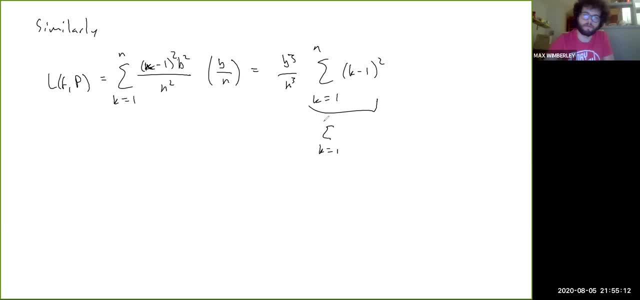 um, as the sum from k equals one to n of or to n minus one of k, squared right, because um, uh, because uh, the first term is zero, so, uh, so we can eliminate the first term and then, like, shift all the indices, uh, so this is so this, this is like whatever you get by putting in n minus one. 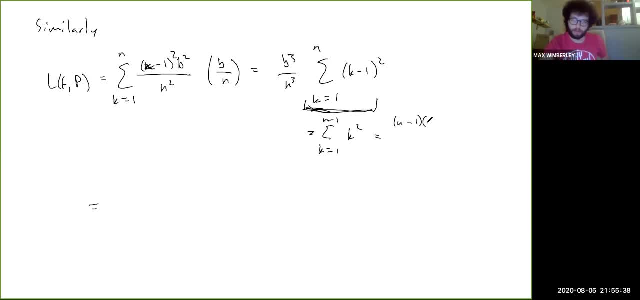 so this is like n minus one times n times two, n minus one over six. so overall we have b cubed over n cubed uh times n minus one, n 2n minus 1 over 6. so l of f is greater than or equal to b cubed over n cubed times n minus 1. 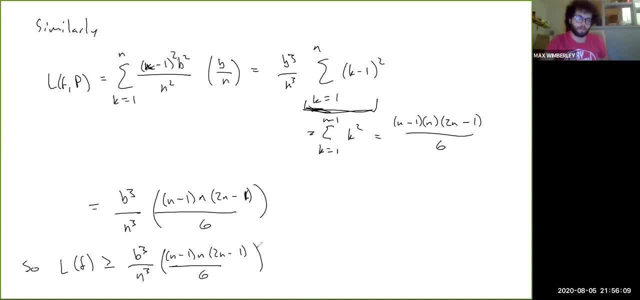 n, 2n minus 1 over 6, and then this tends, as n goes to infinity, to again b cubed over 3, so l of f is greater than or equal to b cubed over 3. but then since, well, let's see, yeah, so. 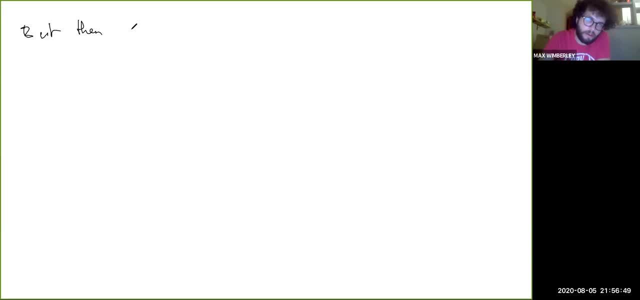 yeah, from this, so we can conclude that l of f equals u of f, um, so, okay, well, all right. okay, this is this relies on. okay, so we haven't proved this yet. we will soon show that l of f is always less than or equal to u of f. 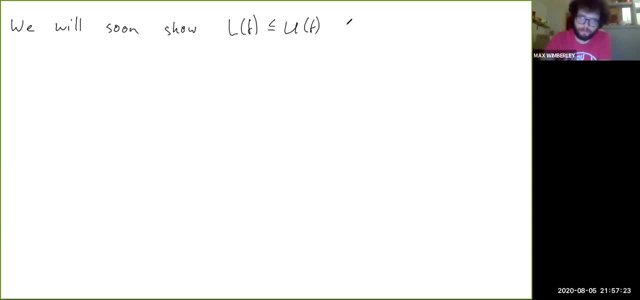 okay, so any any bounded function on any interval, you always have that l of f is less than or equal to u of f. this is not actually obvious from what we've done so far, and i'll explain more about that when we get to proving it, but so um so, since l of f is greater than or equal to b cubed over 3, and u of f is less, 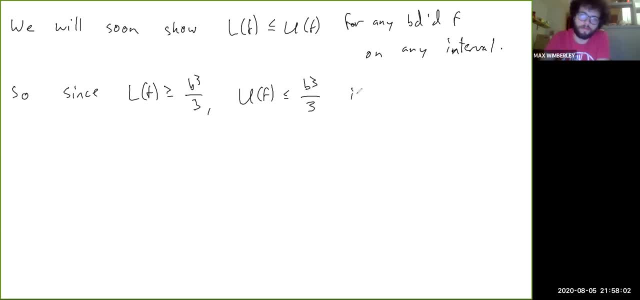 than or equal to b cubed over 3. in this case, for example, um f of x equals x squared is integrable on 0b. here and times u of f is less than or equal to u of f and u of f is, and, as we expected, the integral from 0 to B of F. sorry, let me make that F look. 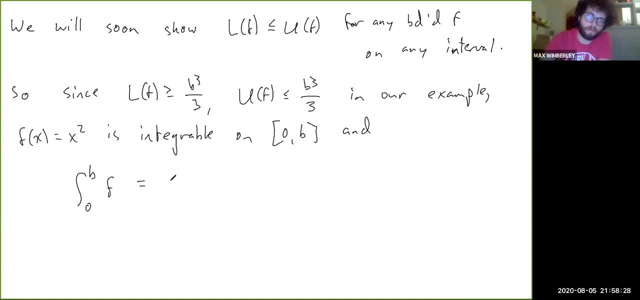 a little bit better. so this equals B cubed over 3. okay, because L of F this. this implies that L of F is greater than or equal to U of F, but we already know that L of F is less than or equal to U of F, so they have to be equal right and 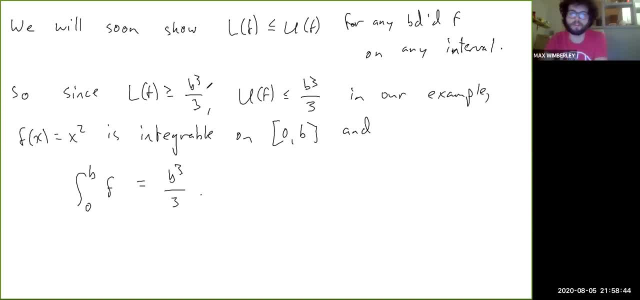 in particular, they have to equal this common bound here. okay, so that's a. that's an example of an integrable function. real quick, let's also look at an example of a non integrable function. so, yeah, yeah, so 1 for X- the rational numbers, and 0 if X is. 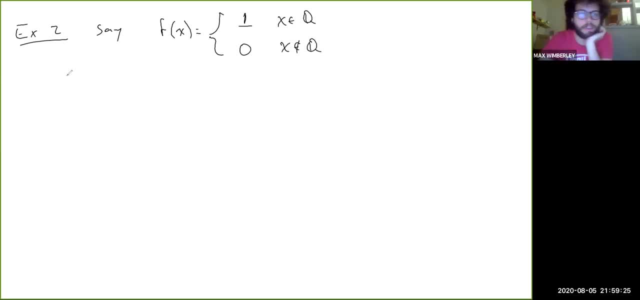 not rational, right on some interval a, b. then for any T, K, T, K minus 1, T K, okay, subset of AB, right, with TK minus 1, less than or less than strictly less than TK, right. we never allow for TK minus 1 to equal TK. then the capital M upper you. 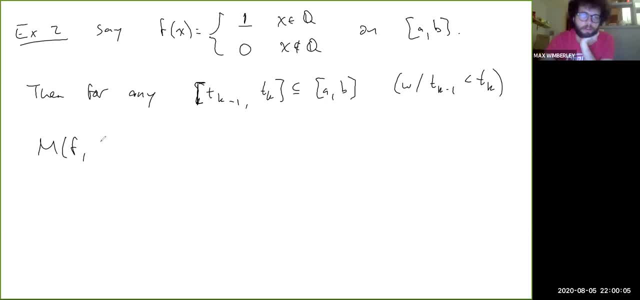 know the upper value of F on this interval is 1 and the lower value of F is 0. so for any P you F, P equals the sum from K, Q equals 1 to N of just 1 times TK minus TK minus 1 right and this sum 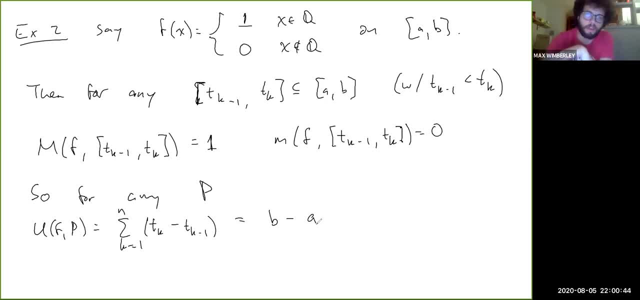 obviously is just the length of the interval. so you get B minus a, which is greater than 0, and so we're assuming that a is strictly less than B, right. and then L of FP equals the sum from K equals 1 to n of 0 times TK, right.